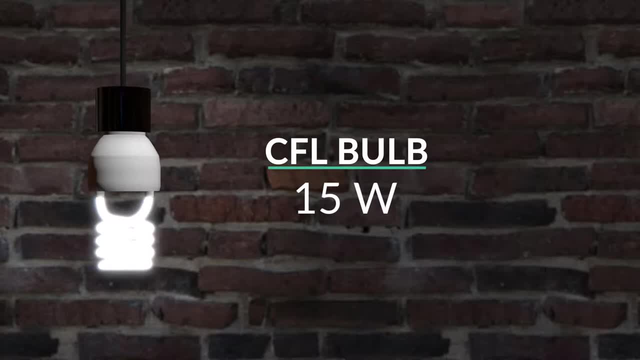 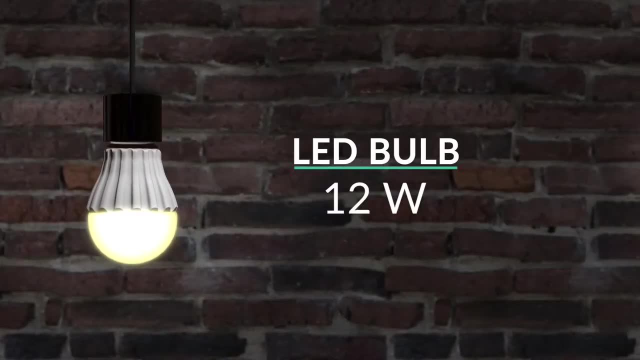 To get the same brightness. this compact fluorescent light bulb, or CFL bulb, uses 15 watts or 15 joules of energy per second. This light-emitting diode light bulb, or LED bulb, also has the same brightness and only uses 12 watts or 12 joules of energy per second. 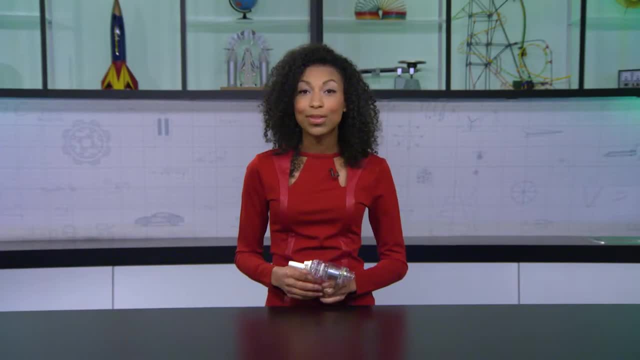 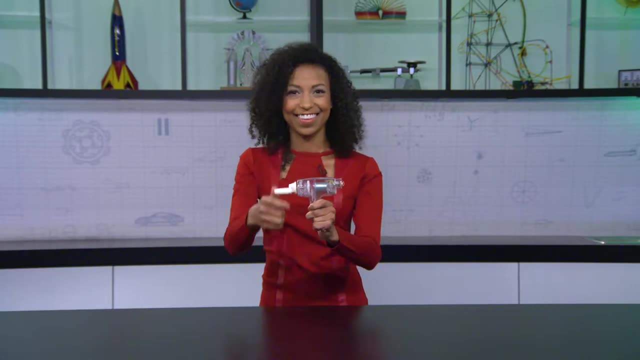 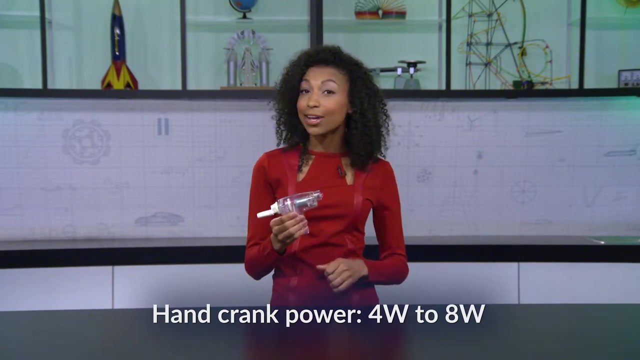 Also, we can turn our own power into electrical power. Using this hand crank, we can produce between 4 watts and 8 watts, or 4 to 8 joules of energy per second. Using this hand crank, we can turn our own mechanical power. 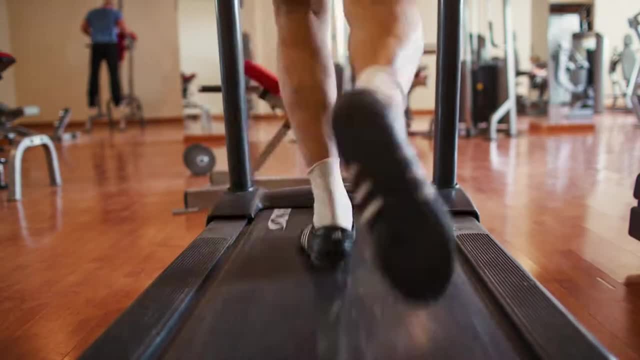 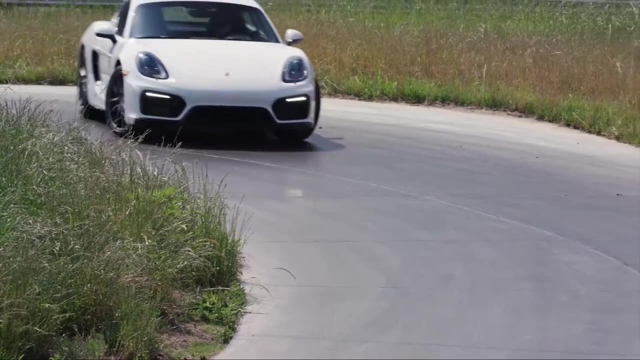 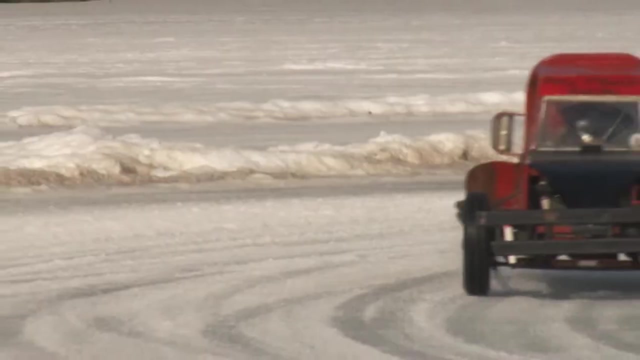 into electrical power. Power is all around us. as humans, We burn watts or joules per second just being alive. These speeding cars on the track are burning watts too. How much depends on a variety of conditions. It's velocity, road conditions, weather conditions, whether it's going up or downhill, things like that. 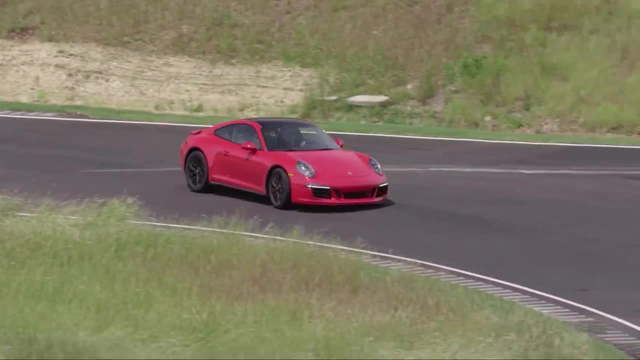 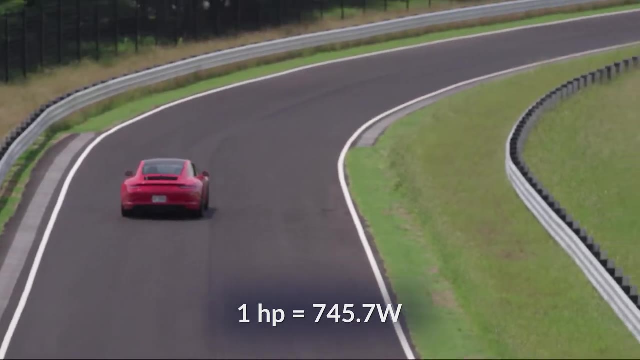 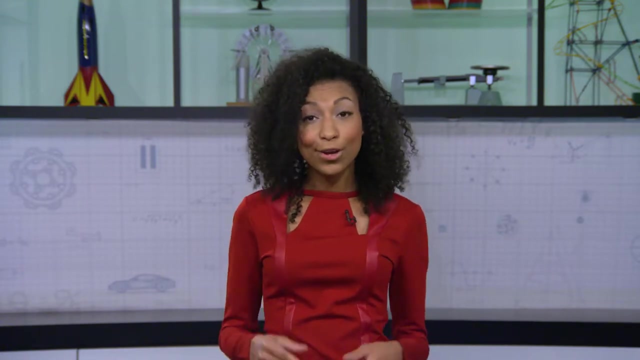 When we talk about motorized engines in America, we use the term horsepower instead of watts. One horsepower is 745.7 watts. Now that you know that power is work divided by time, we can combine these concepts to other formulas. you know to figure out a few things. 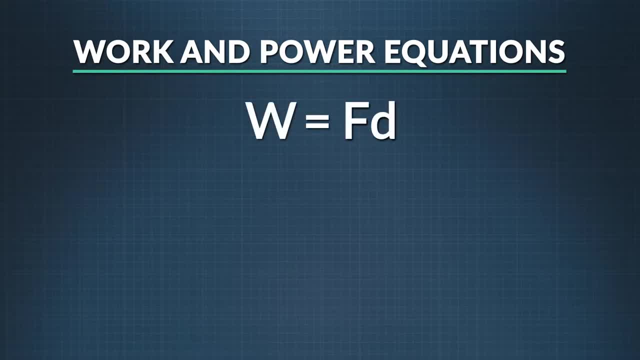 When you combine the equation for work and the equation for power, you can see that power equals force times displacement divided by time. Do you remember what displacement divided by time equals Velocity? So now we have another equation to figure out power. Power is equal to force times velocity. 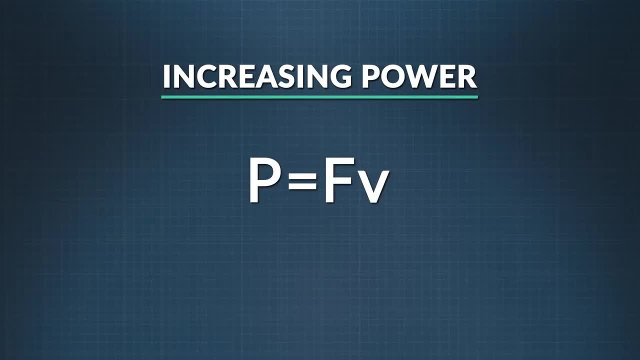 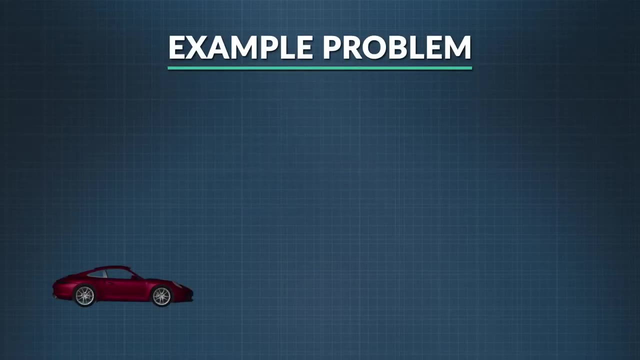 Looking at these relationships shows me ways to increase power. We can get more power when you increase the force exerted by an object. Increasing my velocity also increases my power. Here's a challenge for you. See if you can solve it using the information you just learned. 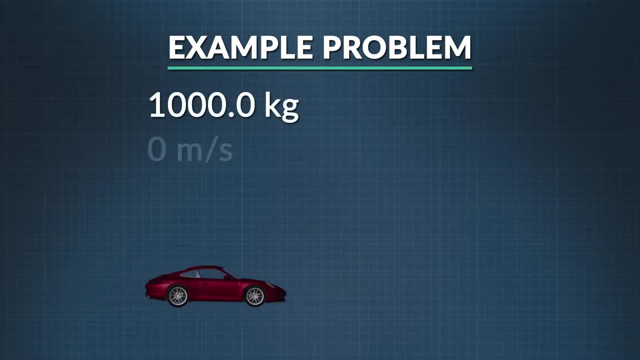 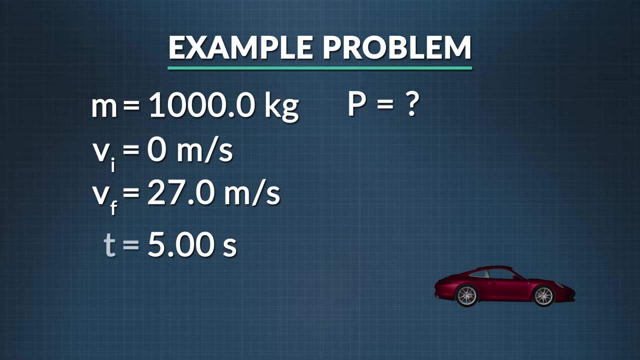 A 1000.0 kilogram car accelerates from 0 to 27.0 meters per second in 5.00 seconds. How much power is the car using to do that? What we know is the mass, the final velocity, the initial velocity and time.